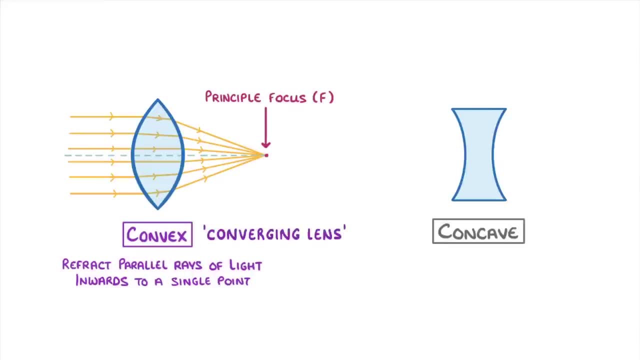 for a convex lens is a converging lens, because they cause the light rays to converge, which just means to come together. Concave lenses, on the other hand, cave in on either side, which causes them to refract parallel rays outwards, so effectively disperse the light. 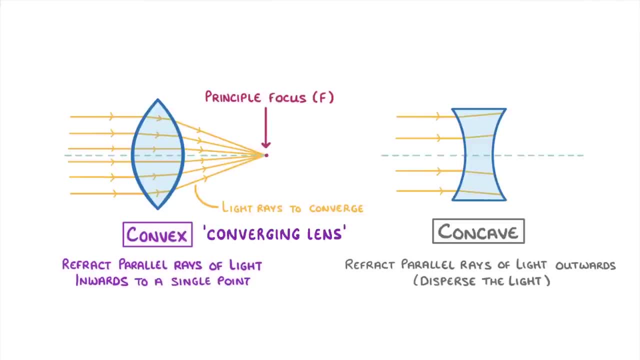 To figure out the direction that they'll be refracted in, we have to trace virtual lines from the lens's principal focus to where the rays hit the lens And then, if we continue these lines, it shows us where the real rays will go. 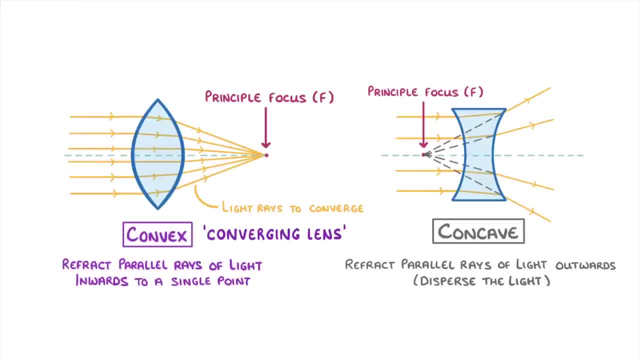 Now, regardless of what type of lens it is, all lenses have a principal focus on both sides and there'll be equal distances from the centre. So our convex lens would also have a principal focus over here, and the concave lens would also have one here. And 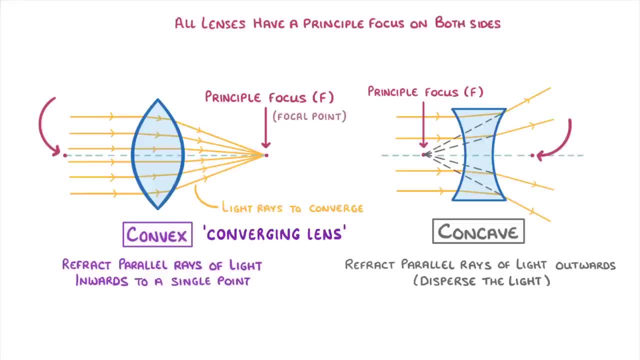 also, you might sometimes hear the principal focus being called the focal point, but they're both exactly the same thing Because they have a principal focus on both sides. lenses are basically symmetrical and can work both ways. So if we were to reverse the direction of the light so that it's travelling, 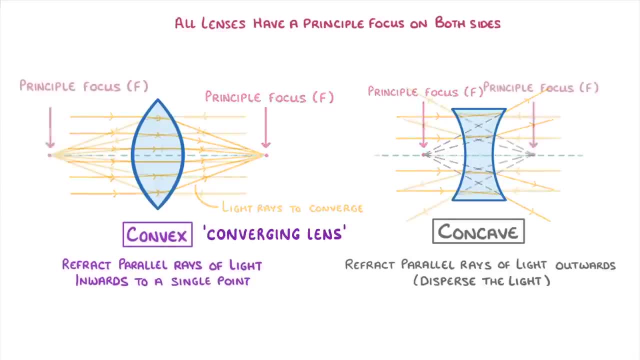 from right to left. everything basically flips and the light focuses on the opposite side of the lens. Another important thing about the principal focus is that it will always sit on the axis, which is this line passing through the middle of the lens, The distance between the principal. 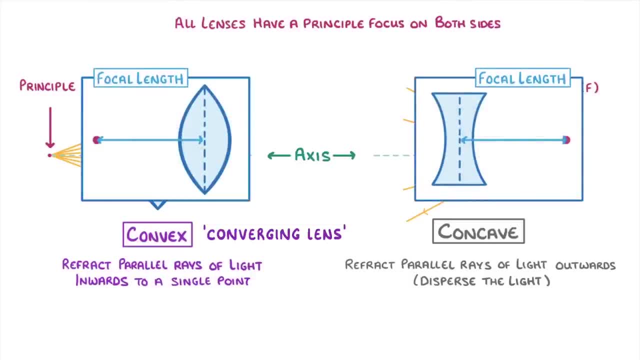 focus and the very centre of the lens is called the focal length, And the shorter the focal length is, the more powerful the lens will be, which just means that it will refract light more strongly. In order to make a lens more powerful, we need to either make it more curved or we 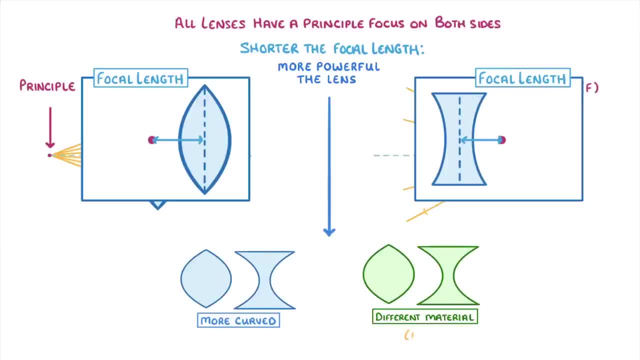 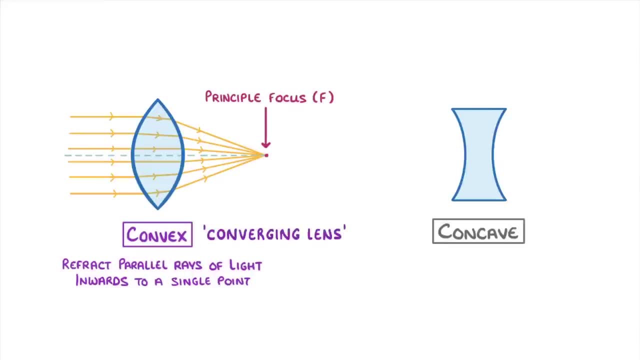 for a convex lens is a converging lens, because they cause the light rays to converge, which just means to come together. Concave lenses, on the other hand, cave in on either side, which causes them to refract parallel rays outwards, so effectively disperse the light. 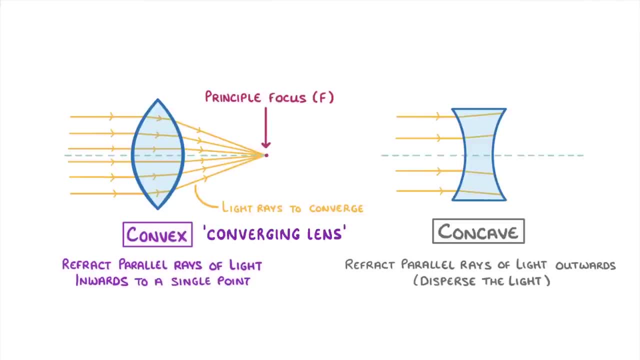 To figure out the direction that they'll be refracted in, we have to trace virtual lines from the lens's principal focus to where the rays hit the lens And then, if we continue these lines, it shows us where the real rays will go. 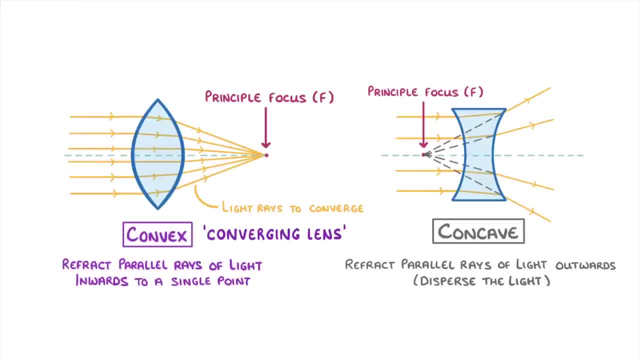 Now, regardless of what type of lens it is, all lenses have a principal focus on both sides and there'll be equal distances from the centre. So our convex lens would also have a principal focus over here, and the concave lens would also have one here. And 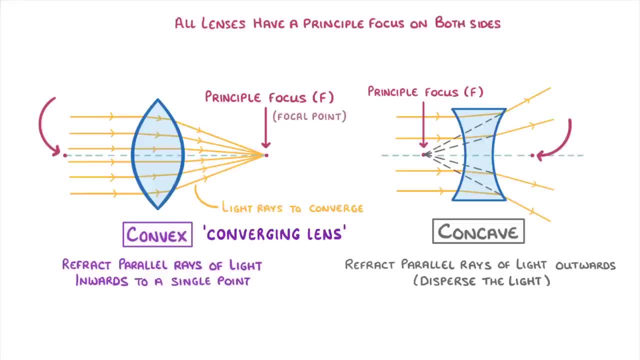 also, you might sometimes hear the principal focus being called the focal point, but they're both exactly the same thing Because they have a principal focus on both sides. lenses are basically symmetrical and can work both ways. So if we were to reverse the direction of the light so that it's travelling, 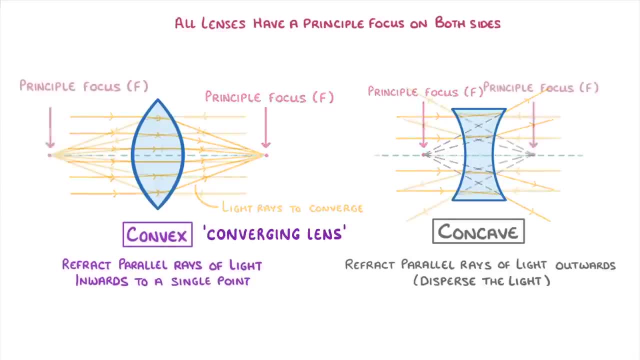 from right to left. everything basically flips and the light focuses on the opposite side of the lens. Another important thing about the principal focus is that it will always sit on the axis, which is this line passing through the middle of the lens, The distance between the principal. 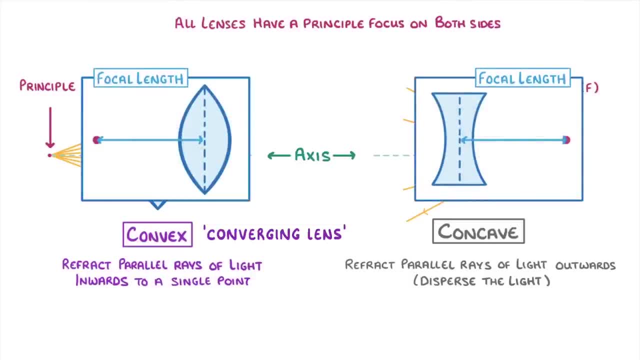 focus and the very centre of the lens is called the focal length, And the shorter the focal length is, the more powerful the lens will be, which just means that it will refract light more strongly. In order to make a lens more powerful, we need to either make it more curved or we 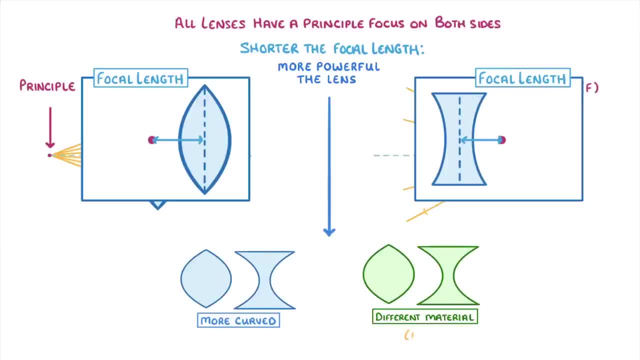 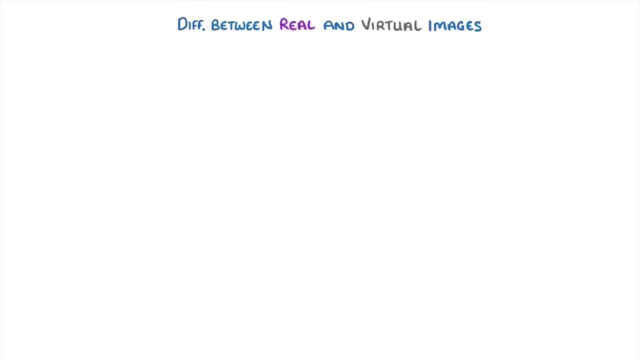 The last thing we need to cover is the difference between real and virtual images, which, to be honest, is kind of a weird concept. so just bear with us and hopefully it'll make sense Now. regardless of whether it's real or virtual, images are formed at points where all the 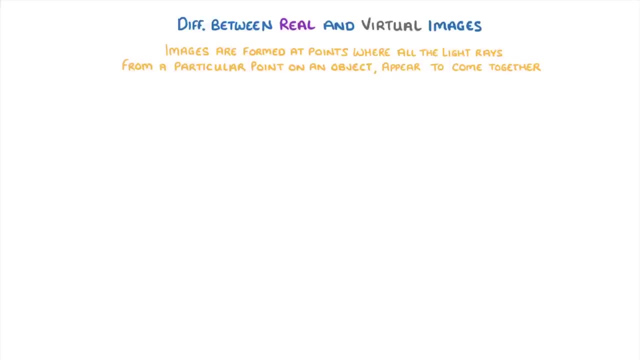 light rays from a particular point of view are reflected. A real image, like we can see here, is formed when the light rays actually do come together to form the image. For example, these light rays from the chicken's head pass through the lens and converge in. 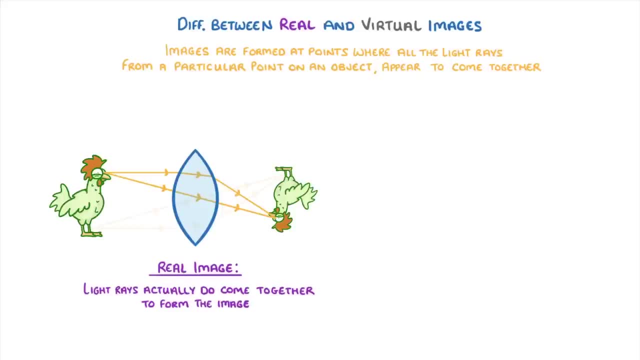 the bottom right, which is why we see the chicken's head down at the bottom. Meanwhile, the light rays from the feet converge in the top right, and so we see the feet at the top. And because it's a real image, if there was a screen here, then the image could be captured. 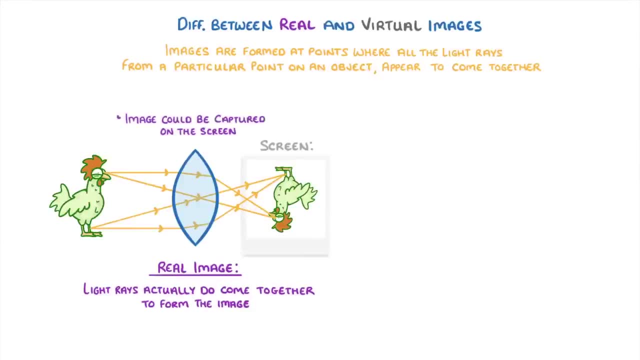 on the screen To give you some idea of where this happens in real life. whenever you look at a real life object like a spanner, the light rays from that object pass through the lens in your eye and form a real image on your retina. 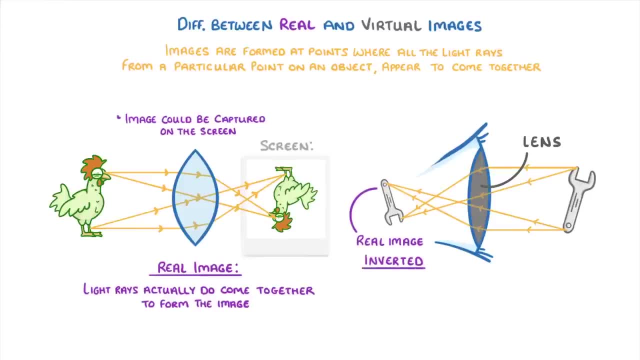 And it is actually inverted like this one here. We just don't notice it, Because our brain corrects it for us so that everything appears to be the right way up. If we look at this diagram, instead, though, we're seeing a virtual image. 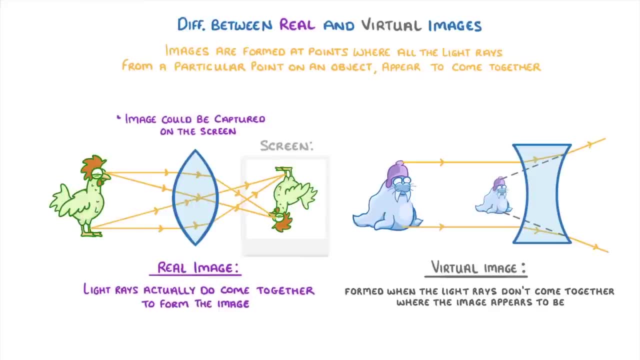 Virtual images are formed when the light rays don't actually come together where the image appears to be. For example, in this case, these dashed lines aren't actually light rays, they're just virtual rays. They're rays that we trace back from these points towards the focal point. 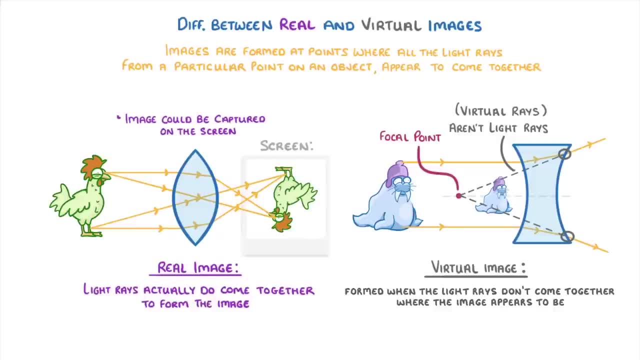 So, because these are only virtual rays, what we're forming is only a virtual image. The most common example of a virtual image is whenever you look in the mirror, The images you see aren't real images Because, although the images appear to be behind the mirror, there can't really be any rays. 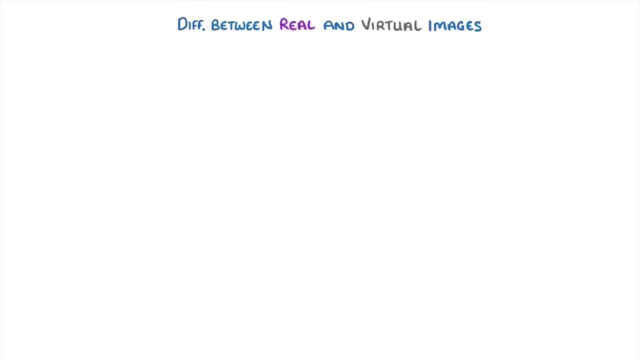 The last thing we need to cover is the difference between real and virtual images, which, to be honest, is kind of a weird concept. so just bear with us and hopefully it'll make sense Now. regardless of whether it's real or virtual, images are formed at points where all the 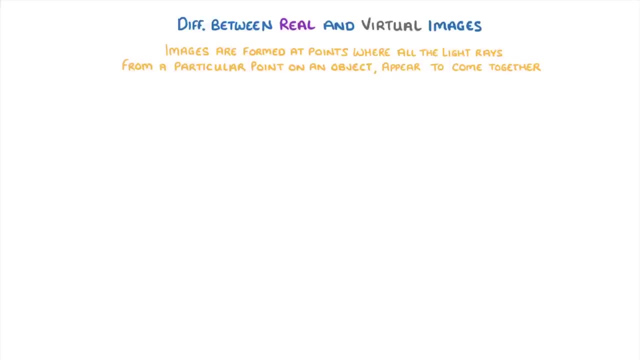 light rays from a particular point of view are reflected. A real image, like we can see here, is formed when the light rays actually do come together to form the image. For example, these light rays from the chicken's head pass through the lens and converge in. 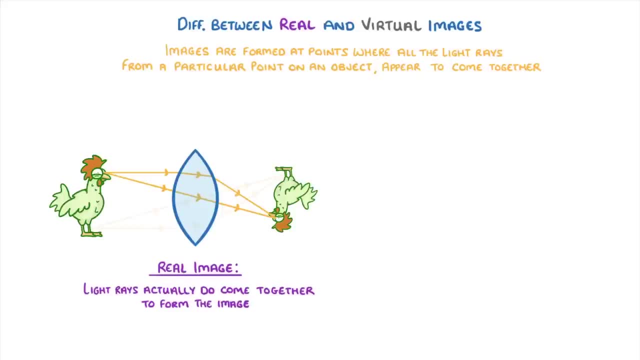 the bottom right, which is why we see the chicken's head down at the bottom. Meanwhile, the light rays from the feet converge in the top right, and so we see the feet at the top. And because it's a real image, if there was a screen here, then the image could be captured. 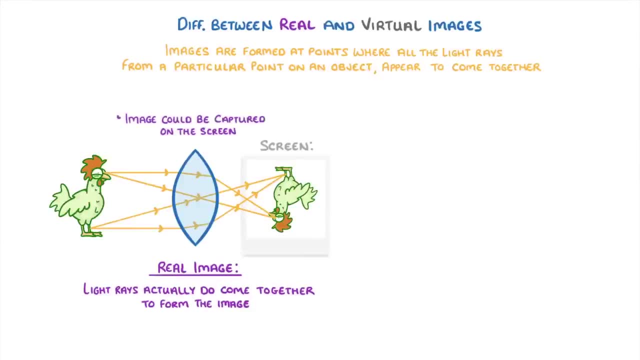 on the screen To give you some idea of where this happens in real life. whenever you look at a real life object like a spanner, the light rays from that object pass through the lens in your eye and form a real image on your retina. 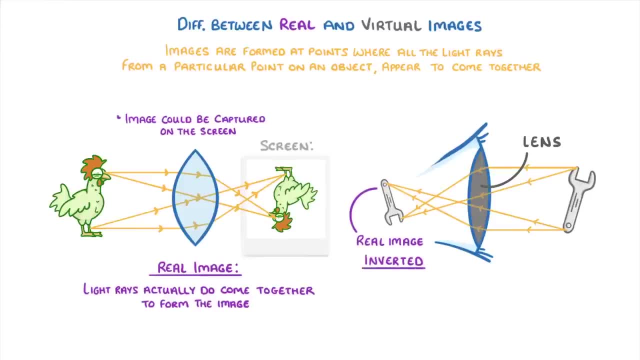 And it is actually inverted like this one here. We just don't notice it, Because our brain corrects it for us so that everything appears to be the right way up. If we look at this diagram, instead, though, we're seeing a virtual image. 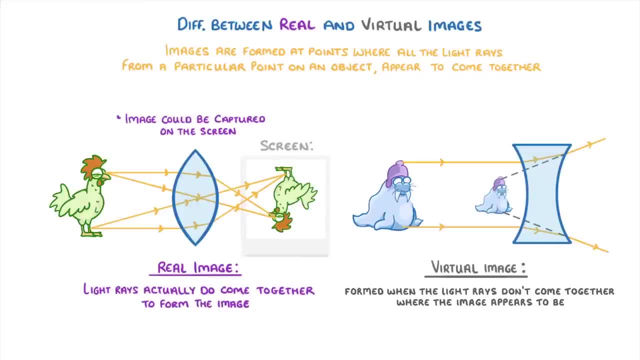 Virtual images are formed when the light rays don't actually come together where the image appears to be. For example, in this case, these dashed lines aren't actually light rays, they're just virtual rays That we don't see. We trace back from these points towards the focal point. 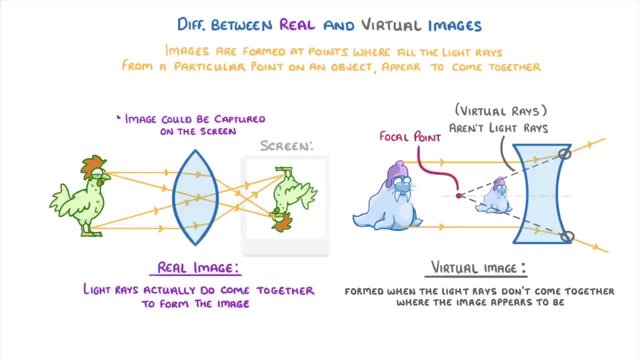 So, because these are only virtual rays, what we're forming is only a virtual image. The most common example of a virtual image is whenever you look in the mirror, The images you see aren't real images Because, although the images appear to be behind the mirror, there can't really be any rays.